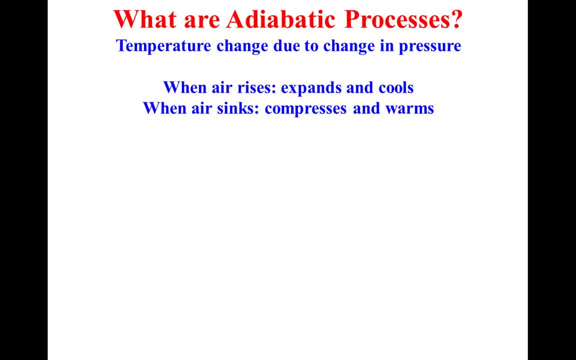 In the last part of this week's lab we're going to be looking at how temperature of an air mass changes as it's forced to rise up and over a mountain range. Those temperature changes as air rises and sinks occur as a result of what are known as adiabatic processes. Temperature changes that occur as a result of a change in pressure. As you rise, pressure is decreasing. In other words, as you move up to higher elevations in the atmosphere, the air pressure decreases. That allows air to expand as it rises. 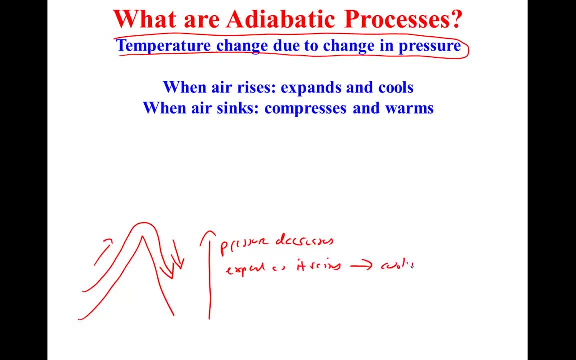 And this causes cooling, Adiabatic cooling. Cooling not due to a loss of heat, but cooling due to a loss of pressure and an expansion in volume. So when air rises, it encounters lower pressures, expanding as it does so And cooling adiabatically as a result. 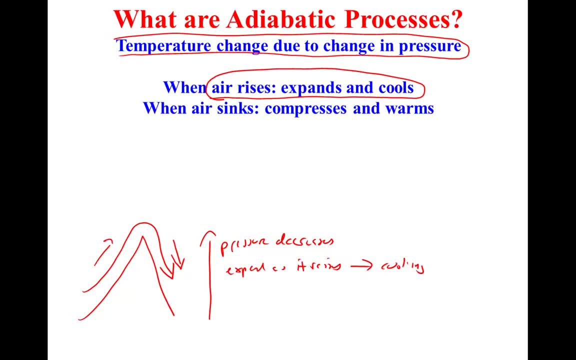 The opposite is true when air sinks. When air sinks, it encounters lower pressures. When air sinks, it encounters higher pressures. This compresses the air, Volume decreases And temperature warms as a result. That warming again is not due to an addition of heat, but is occurring due to a change in pressure and volume. 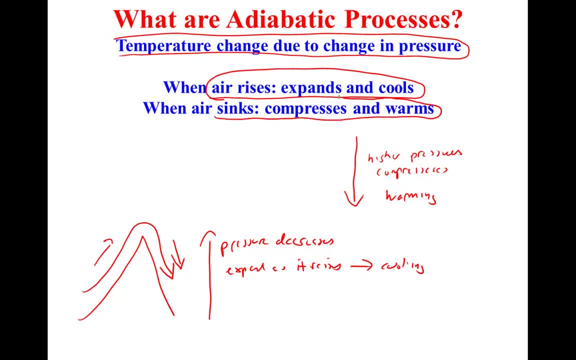 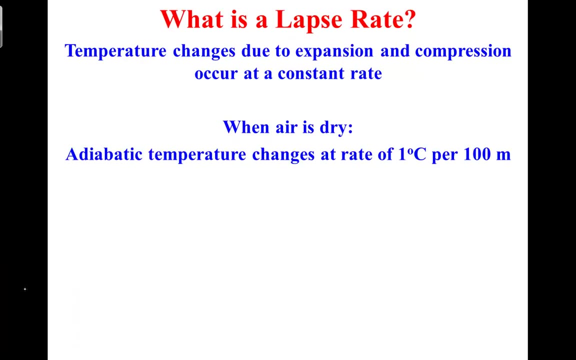 As air sinks and encounters higher pressures, that air is compressed into a smaller volume. that's associated with adiabatic warming of that air. Adiabatic temperature changes. temperature changes due to a change in pressure occur at a constant rate, known as the lapse rate. 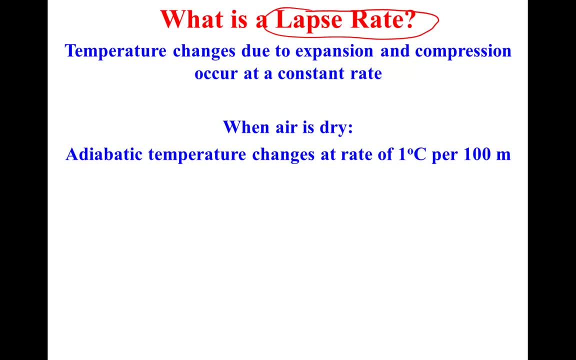 When the air is dry, meaning unsaturated relative humidity less than 100% adiabatic temperature changes occur at the rate of 1 degree Celsius per 100 meters of elevation change. In other words, when dry air rises, it cools at 1 degree C per 100 meters. 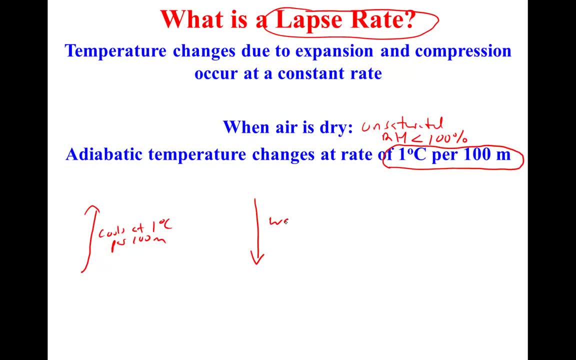 When dry air sinks, it warms. it warms at 1 degree C, at 1 degree C per 100 meters. per 100 meters. Again, this lapse rate is constant so long as the air is unsaturated, so long as the relative humidity 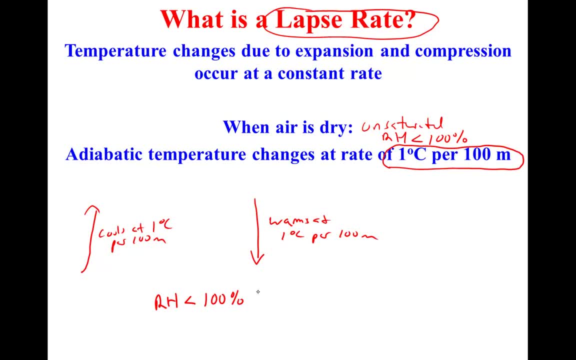 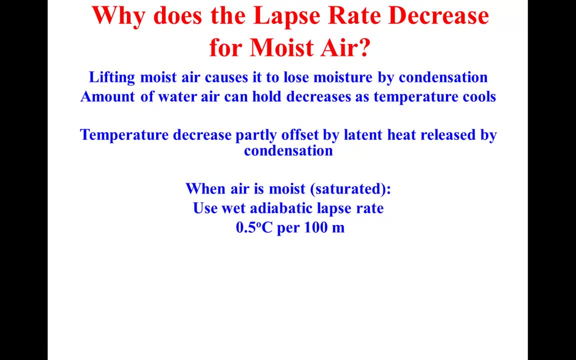 is less than 100%. is less than 100%, However, the lapse rate is smaller. when the air mass is moist, In other words, when relative humidity is 100%. temperature change occurs at the wet adiabatic. at the wet adiabatic. 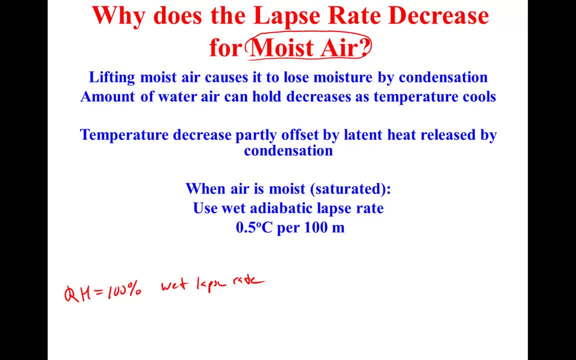 lapse rate. Wet adiabatic lapse rate is smaller is smaller than the dry lapse rate lapse rate. This is because the cooling. This is because the cooling from lifting of that air mass is partly offset by latent heat being released as water vapor condenses. 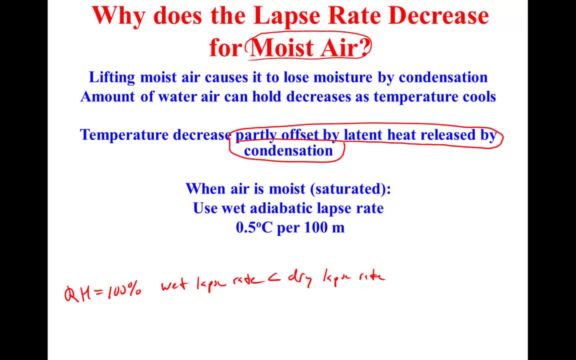 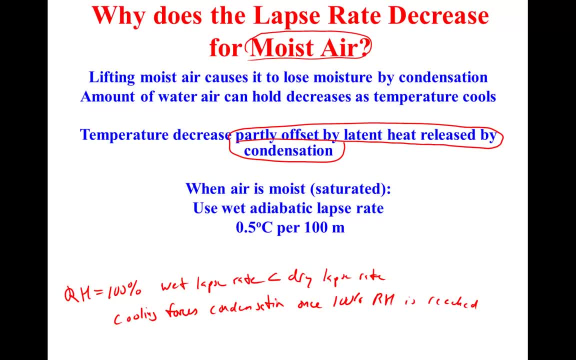 any further. cooling must be accompanied by a loss of water. A loss of water vapor causes precipitation and precipitation, As that water vapor condenses, latent heat is released which partly offsets that latent heat, partly offsets the adiabatic cooling. As a result, 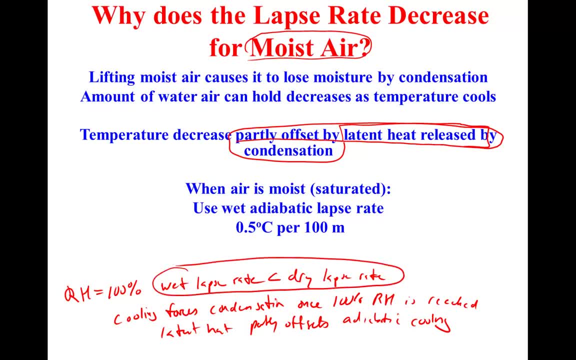 the wet lapse rate is smaller than the dry lapse rate As a function of how much water vapor is being condensed, which is in turn a function of the temperature of that air mass, because air can hold more water at warmer temperatures, releasing more latent heat by condensation. 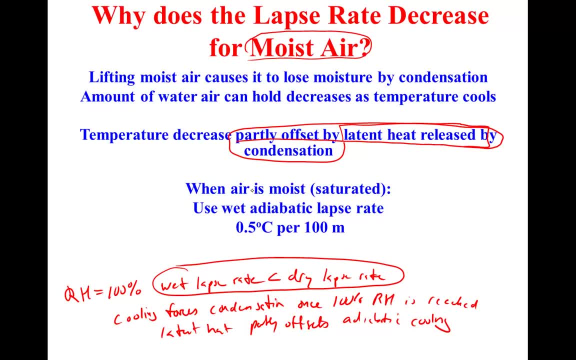 and less water at colder temperatures. So the wet adiabatic lapse rate varies as a function of the amount of condensation that's occurring and the amount of latent heat being released. But a good approximation for the wet adiabatic lapse rate. 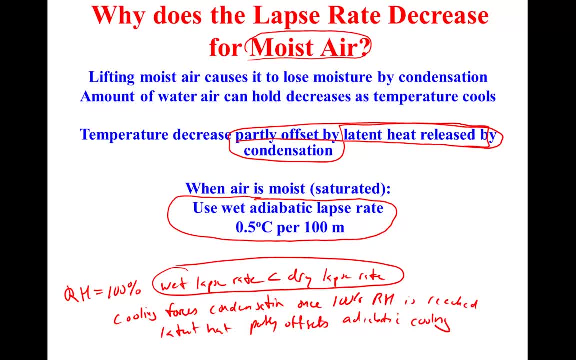 is about half a degree Celsius per 100 meters. If you were to go on and take an advanced atmospheric science class, you would use the actual wet adiabatic lapse rate that varies as a function of the temperature of the air mass. This is reasonable. 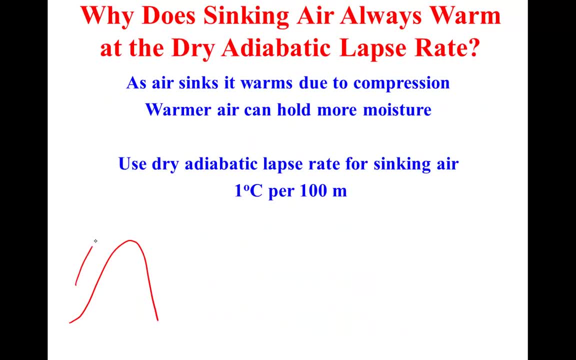 Now, once air gets up and over the mountain, it sinks. And as it sinks it warms, And it always warms at the dry adiabatic lapse rate. This is because as air warms, it can hold more water. In other words, 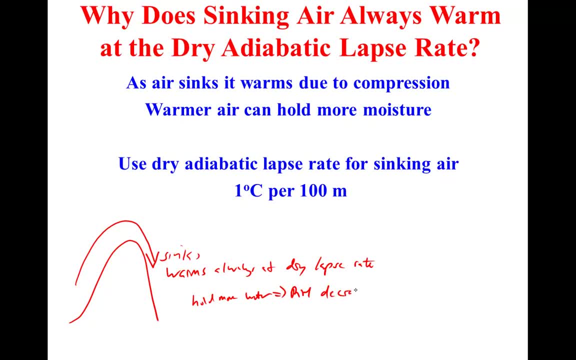 relative humidity is less than 100%. as the air mass warms, Condensation is not occurring. There's no condensation. Relative humidity is less than 100%, So the air mass is warming at the dry lapse rate. Again, the dry lapse rate. 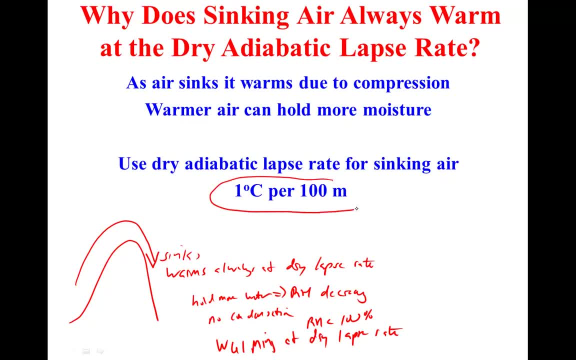 is one degree Celsius per 100 meters per second. So when you lift air, you initially cool at dry rate until 100% relative humidity, Then you cool at the wet lapse rate. once you get over the obstacle, you warm at dry lapse rate. So those are. 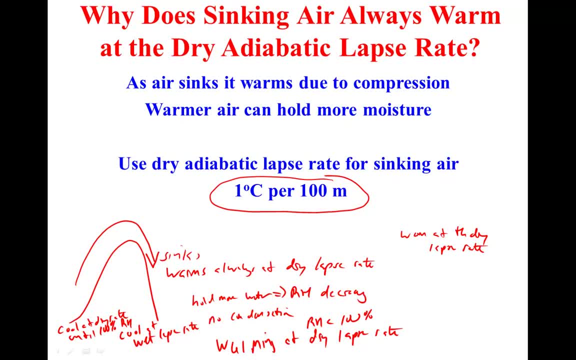 the basic steps in the process. So just to sum up what we've done so far, when we start lifting an air mass, we initially cool at the dry lapse rate, And we do that until we reach 100% relative humidity. At that point we switch. 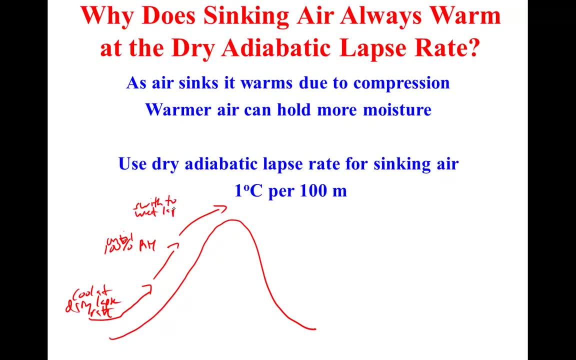 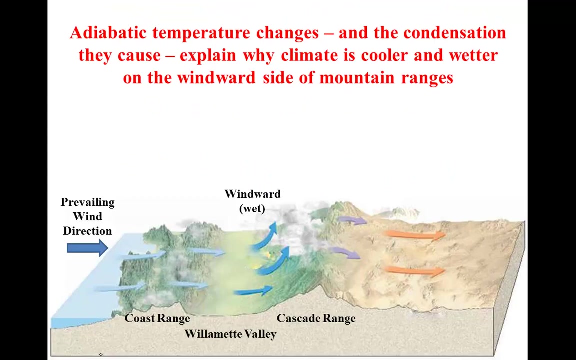 to the wet lapse rate, Which is smaller than the dry lapse rate. Then, as air sinks, we warm at the dry lapse rate Because relative humidity is getting lower and lower and is always less than 100% relative humidity. So these adiabatic 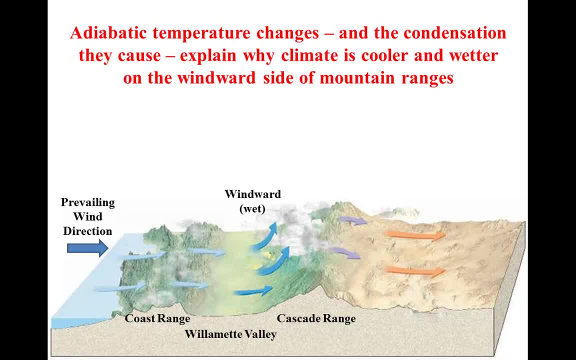 temperature changes and the condensation they cause once 100% relative humidity is reached explains why the climate is both cooler and wetter on the windward side of a mountain range. This is our mountain, and the wind is going west to east and this side. 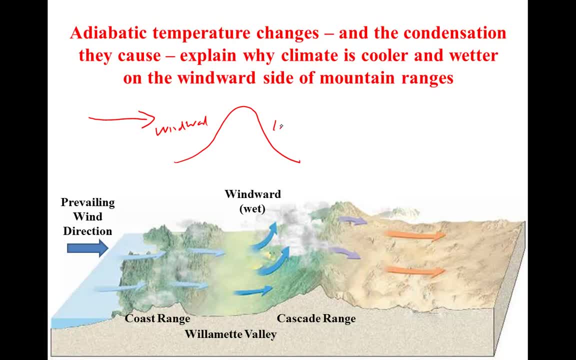 is the windward side and this side is the leeward side, the side opposite the wind. So the windward side is the side of the mountain that faces the prevailing wind direction In Oregon, as is the case elsewhere in the middle latitudes of the earth. 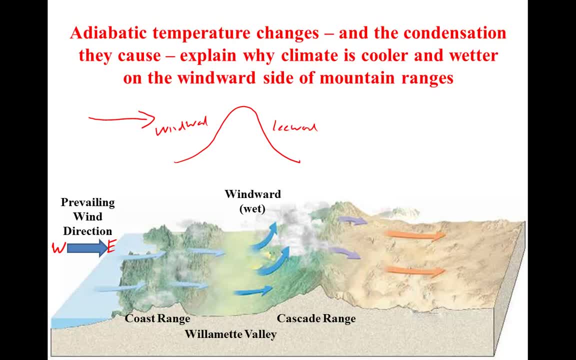 wind is going east. As air moves over Oregon, it rises over two mountain ranges: The coastal range and the cascades. Each time it is forced to rise as it encounters that topographic obstacle causing air, causing air to cool and condense on the windward side. 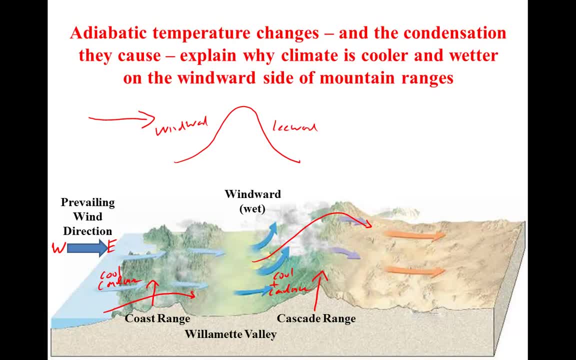 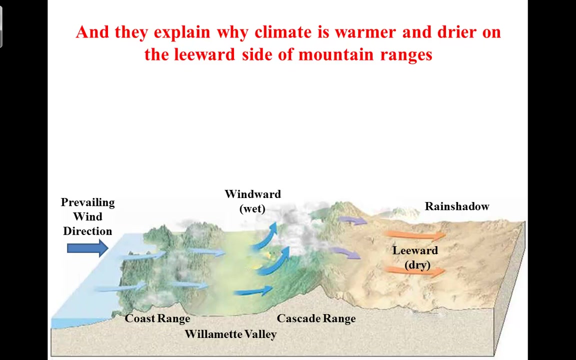 of each of those mountain ranges. This is where most of the precipitation occurs, Again on the side of the mountain ranges that faces the prevailing wind direction. Likewise, adiabatic temperature changes that occur as air sinks on the leeward side of a mountain range. 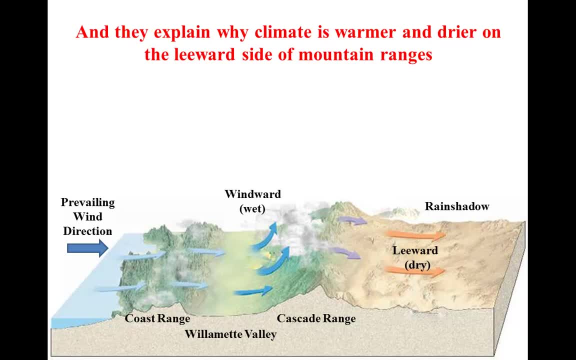 explains why it's warmer, why the climate is warmer and drier on that side of the range, As air sinks. it warms as air sinks and because warmer air has the ability to hold more moisture, we have no condensation occurring, In other words, on the leeward side. 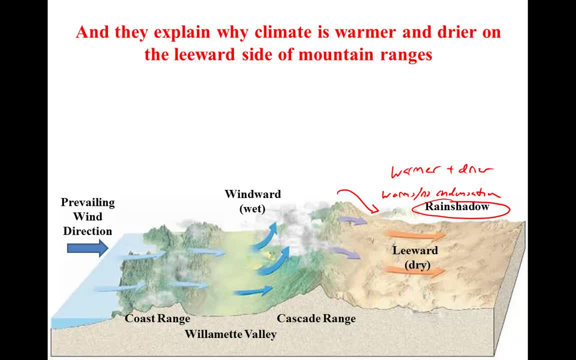 we have a rain shadow. Most of the precipitation fell on the upwind side of the mountain range. This is called the orographic effect, Also called the rain shadow effect. Adiabatic temperature change is occurring as air is forced to rise on the windward side. 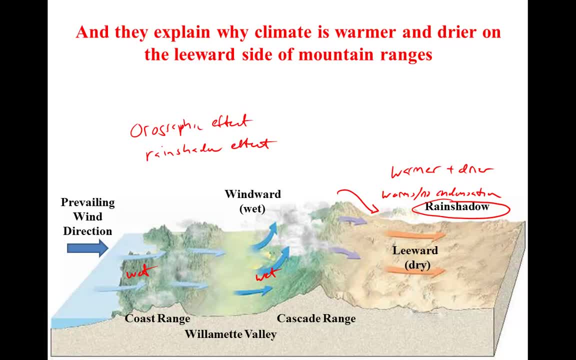 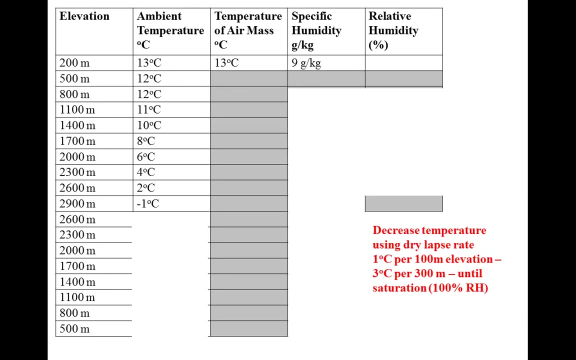 of the mountain, cooling and condensing as it does so, and then warming and drying on the leeward side of the mountain range. Let's do an example problem like the one in your lab. Again, we're going to initially cool at the wet lapse rate. 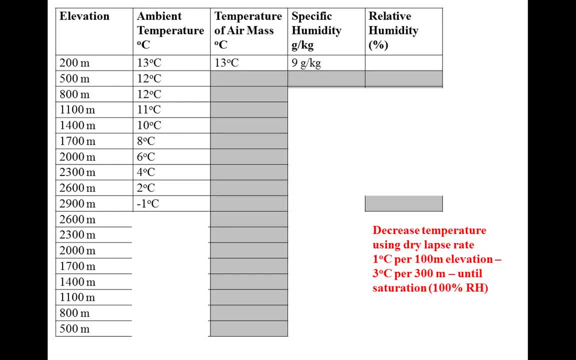 until 100% relative humidity is reached. We will then switch and cool at the wet lapse rate until we get over the mountain and then allow the wear to warm at the dry lapse rate as it sinks down the other side. We will then use the temperature. 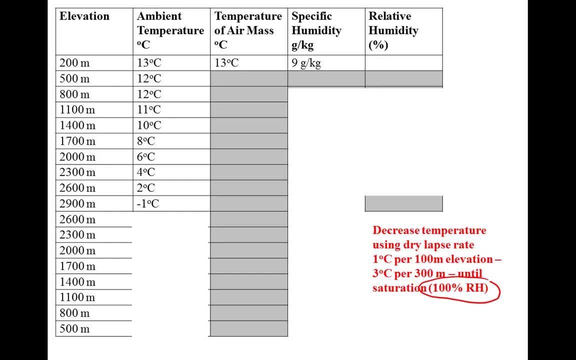 of humidity to decide when to switch from dry to wet lapse rate. So our starting conditions in this sample problem is a temperature of 13 degrees Celsius with 9 kilograms of water per kilogram of air. To calculate relative humidity, we need to know how much water. 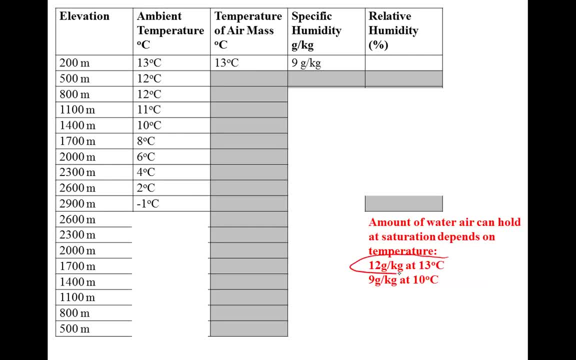 air can hold at different temperatures. Again, these are givens. Air at 13 degrees Celsius can hold 12 grams of water per kilogram of air. Our air actually has 9 kilograms per kilogram. that's its specific humidity, Its relative humidity. 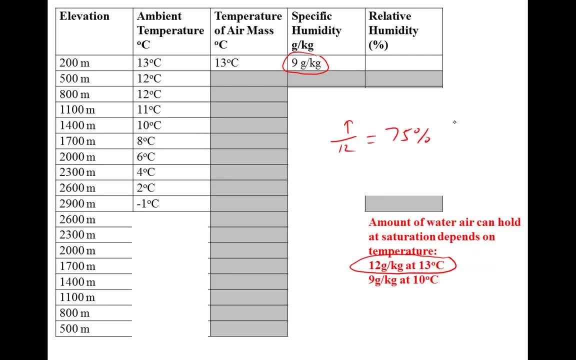 would be 9 divided by 12 times 75 percent. So our air mass has a relative humidity of 75 percent. It has 9 grams of water. It could hold 12 grams. 9 divided by 12 .75 times 100 percent. 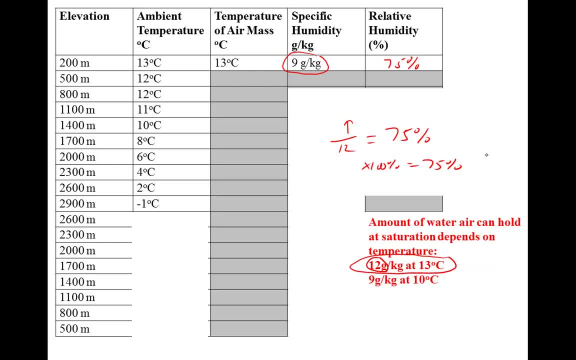 is 75 percent relative humidity. That means we're going to cool our air at the dry adiabatic lapse rate because we're still below 100 percent relative humidity. Dry adiabatic lapse rate: 1 degree per 100 meters or 3 degrees per 300 meters. 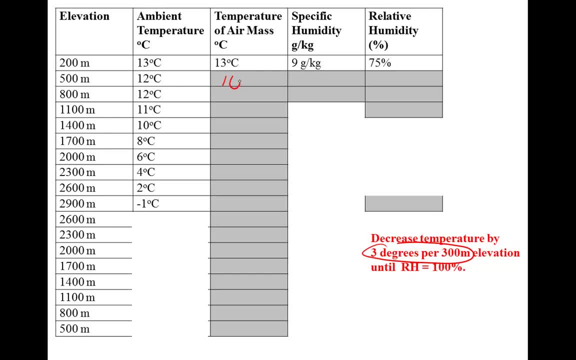 75 percent relative humidity. cool at the dry lapse rate. increase in elevation means our air mass is now at 10 degrees Celsius. Specific humidity remains the same until 100 percent relative humidity is reached. Previously we saw that air could hold 9 grams of water. 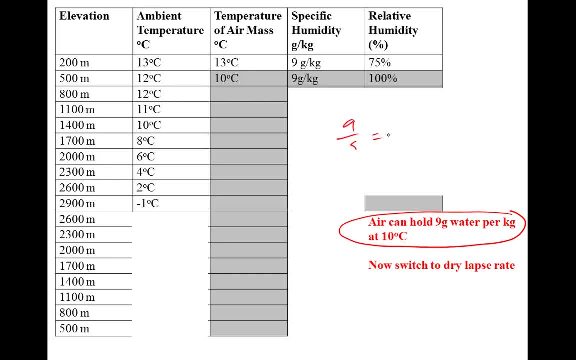 per kilogram at 10 degrees 9 divided by 9 is 1 times 100 percent, 100 percent relative humidity. Now our air mass is saturated. Now we're going to switch to the wet adiabatic lapse rate. The wet adiabatic lapse rate. 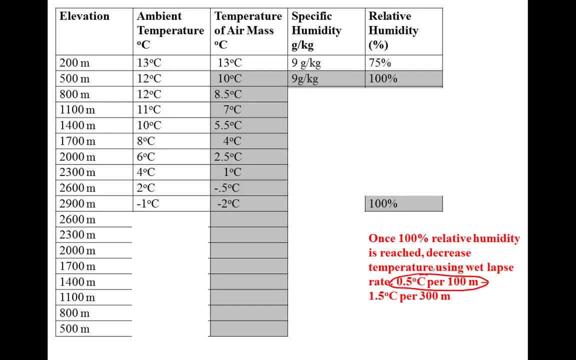 half a degree Celsius per 100 meters approximately, or one and a half degrees Celsius per 300 meters. Once we reach relative humidity, we're going to. we are cooling at the wet adiabatic lapse rate: 8 and a half degrees, 7 degrees. 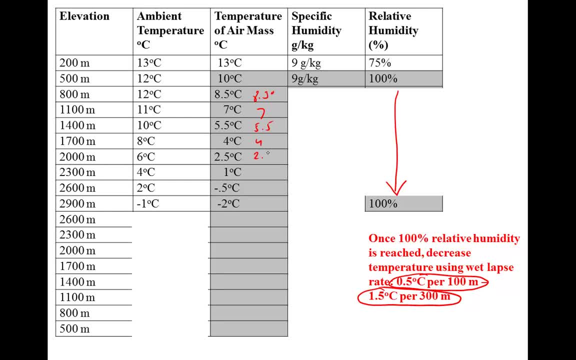 5.5, 4, 2 and a half 1 negative 0.5 and negative 2 degrees Celsius by the time we reach the mountain summit. All this time, relative humidity is 100 percent. Water is being lost by condensation. 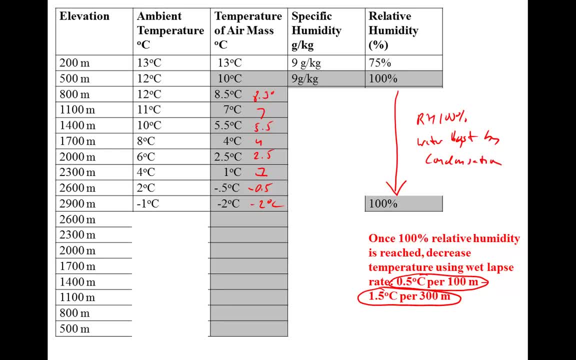 How much water is being lost. we could calculate, but that calculation is beyond the scope of this activity. If you were to take an advanced atmospheric science class, you would calculate how specific humidity changes during wet adiabatic cooling. We're not going to worry. 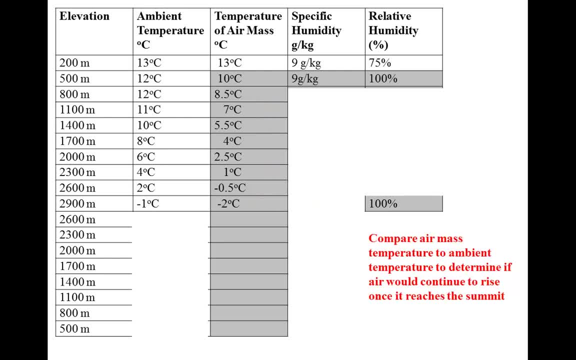 about that today. Once we get to the top of the mountain, we need to compare the temperature of our air to the temperature of the surrounding air to determine if our air mass is going to continue to rise. If the air mass is warmer, we're going to. 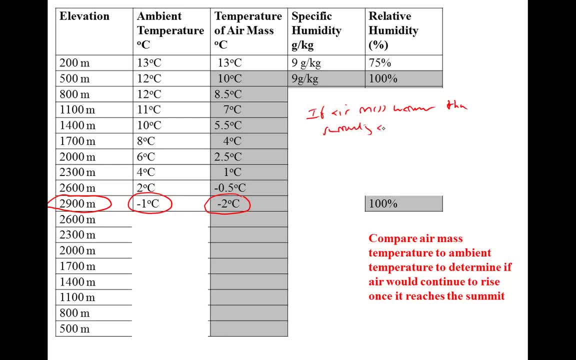 calculate the temperature of our air mass than surrounding air. It will continue to rise even after it's no longer forced to do so by the mountain range, But if the air mass is cooler than the surrounding air, it will stop rising once it runs through the mountain. 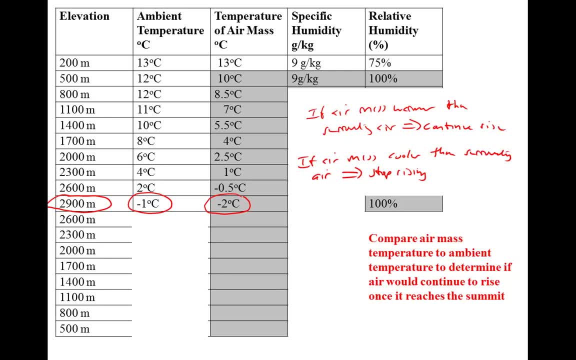 It will stop rising once the terrain no longer forces it to. In this example, our air mass is cooler than the surrounding air, so it's going to stop rising at the top of the mountain and instead start sinking down the other side, warming at the dry lapse rate. 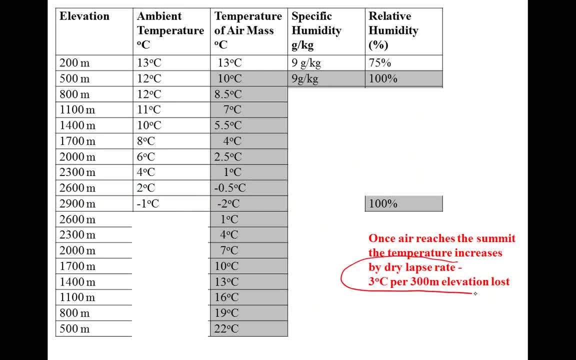 Because when we bring our air mass down the other side, it compresses and warms- warms at the dry lapse rate of 3 degrees C per 300 meters of elevation lost. At the same time, relative humidity is decreasing. you could calculate how much it's decreasing?